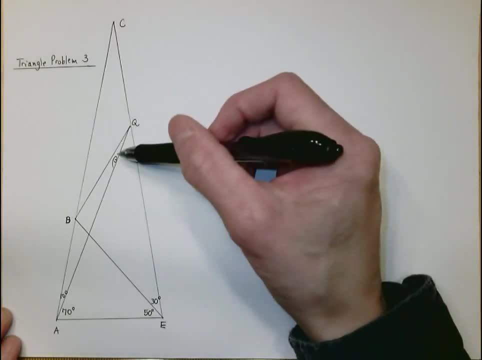 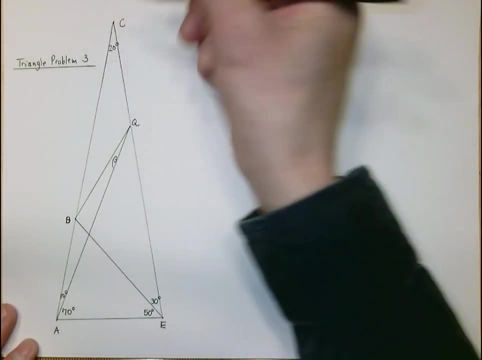 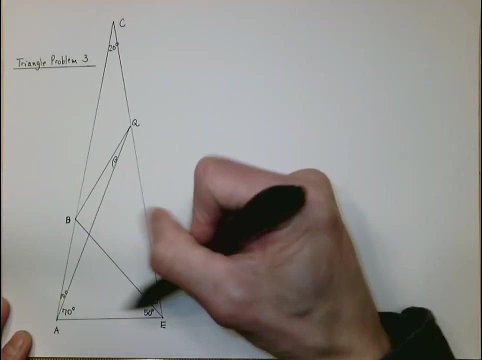 That is 70 degrees, then it's 50 degrees and we are looking for the unknown angle beta. This is 80,, 80, and then we'll make this angle 20 degrees And look at this triangle here: ABE: 50,, 80, and this will be 50 degrees. 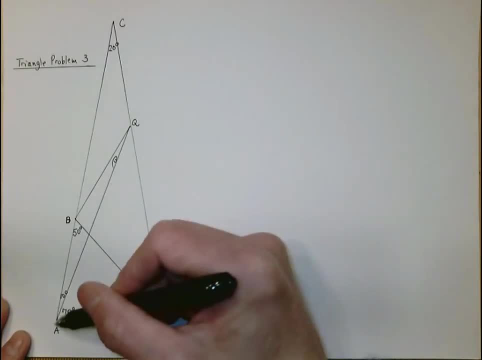 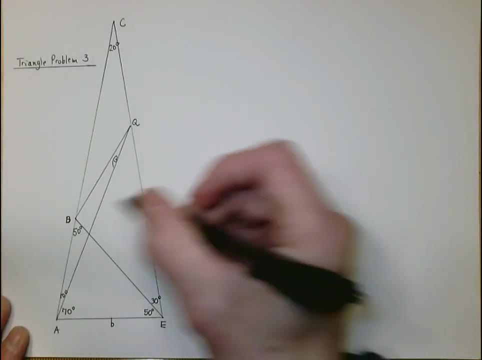 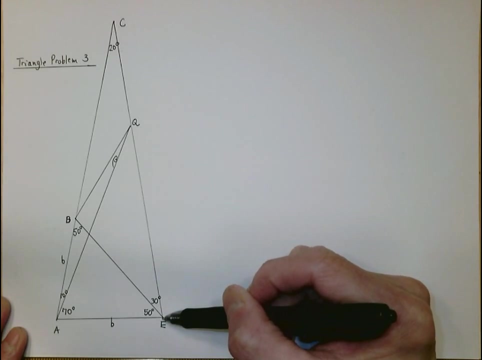 So this is an isosceles triangle, So AB will be congruent to AE, and then we call AE small b And AB will be small b as well, And I'm going to construct an equilateral triangle here with AE the base of the triangle. 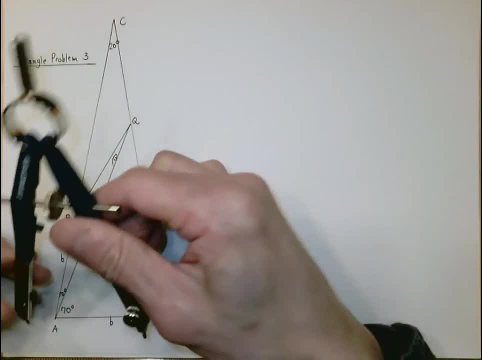 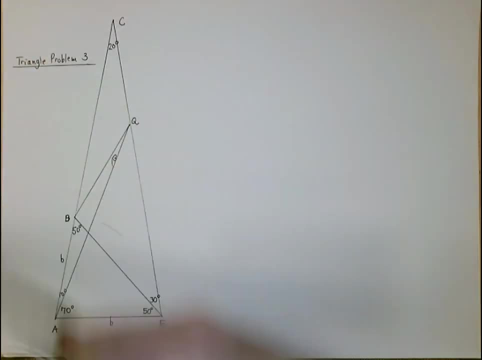 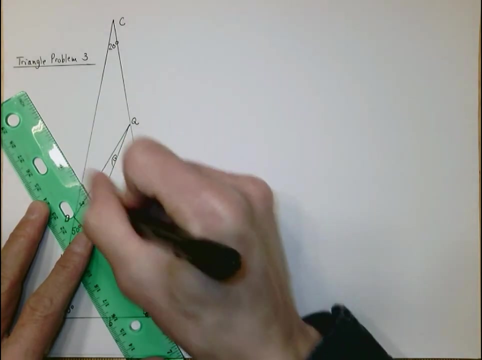 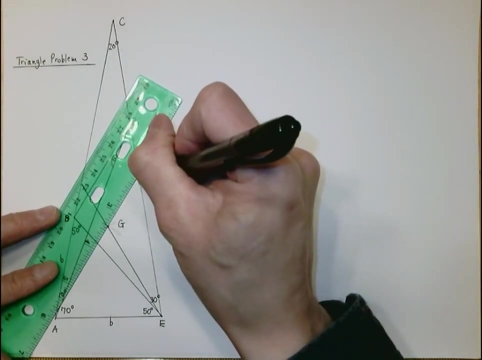 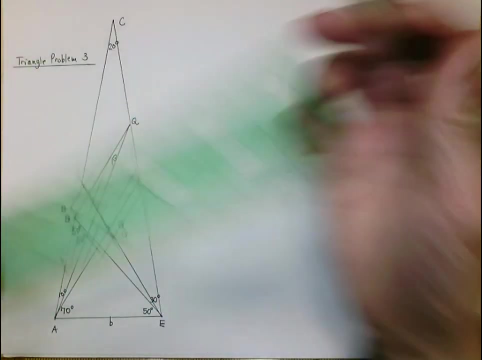 Well, that is not difficult to do. We're going to measure the sermon AE. I'm going to do one more arc. I'm going to call this point G, G to E, and I'm going to connect G to A and I'm going to call this point D. 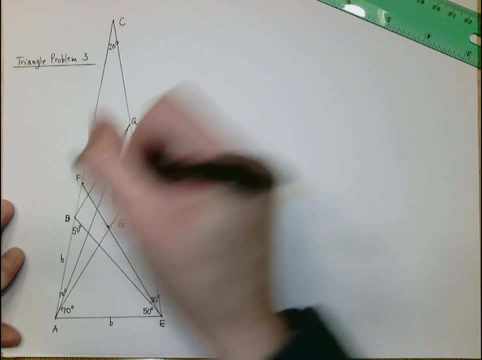 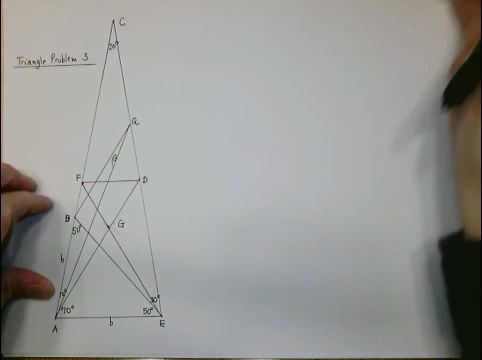 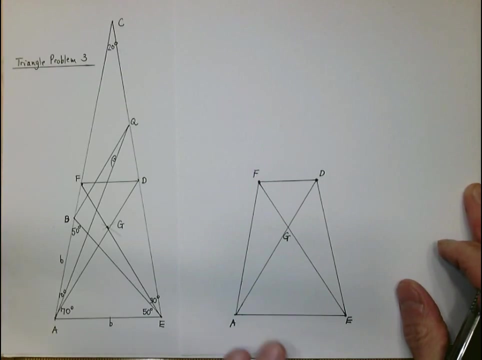 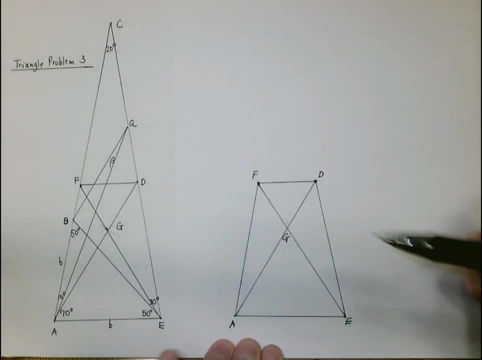 and I'm going to call this point F, I'm going to connect these two points. Well, the next thing is we're going to focus on two triangles here- FGA on the left and DGE on the right- And now we're going to put down what we know. 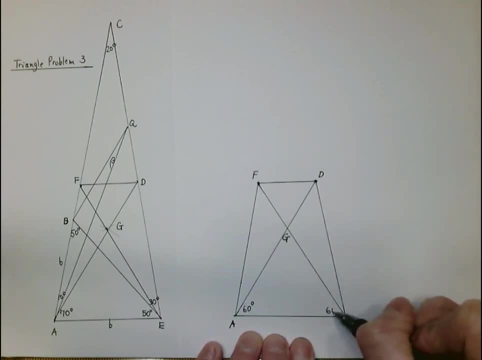 We know that it is 60 degrees. It is 60 degrees, So that is 20 degrees, It is 20 degrees And that is small b. But based on the construction, that is an equilateral triangle, That is small b and that is small b. So that is small b and that is small b. 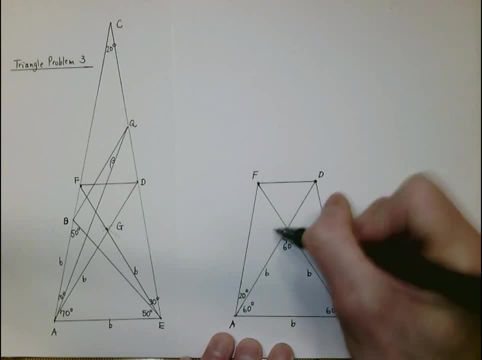 And that is 60 degrees as well. If it is 60, this one will be 120, And that is 120, that is 60, And we can see that the triangle on the left and the triangle on the right are congruent. The reason is quite simple. 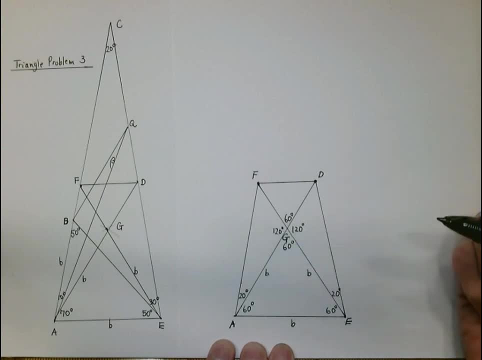 Because we have angle side angle. So these two triangles are congruent And that means that FG will be congruent to GD. But then there's 60 degrees And then there's an isosceles triangle. The sum of these two angles is 120 degrees. 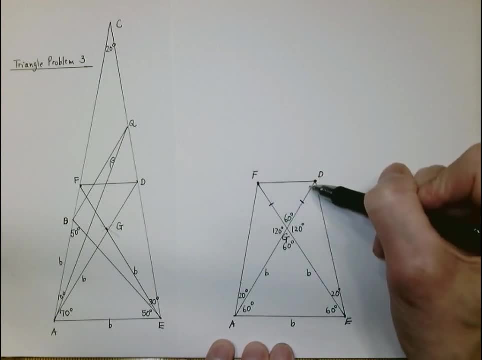 That means F and D must be 60 degrees each, So 60 here and 60 there. So we have another equilateral triangle on the top And I'm going to call this small d And this one will be small d and small d as well. I'm going to transfer the information to the original diagram. 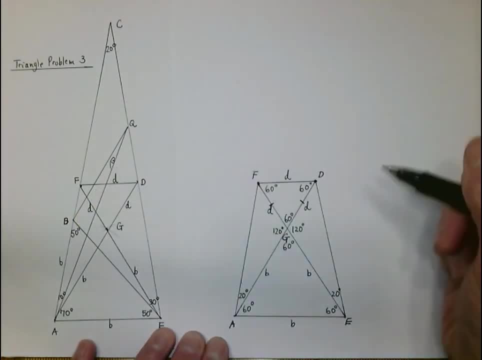 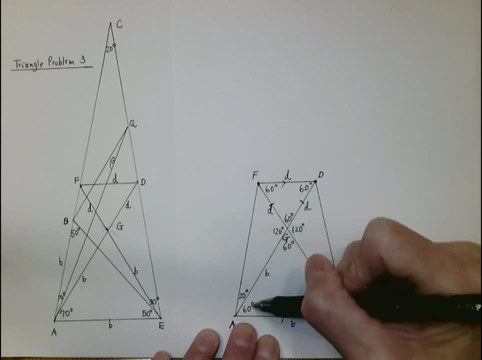 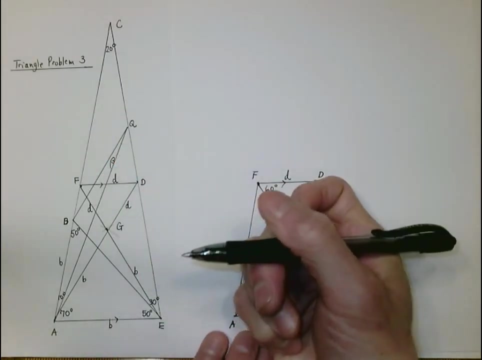 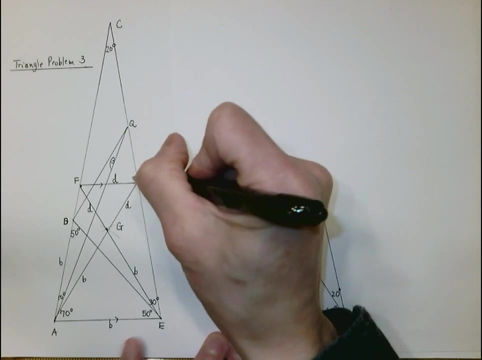 It is d, small d and small d. We also know that these two segments are parallel Because the alternate interior angles are congruent. So these two segments are parallel. If these two segments are parallel, The corresponding angles must be congruent. So this angle will be actually 80 degrees. 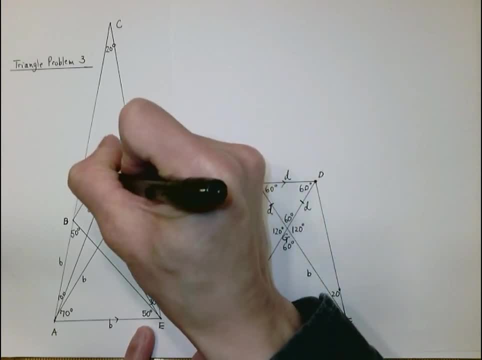 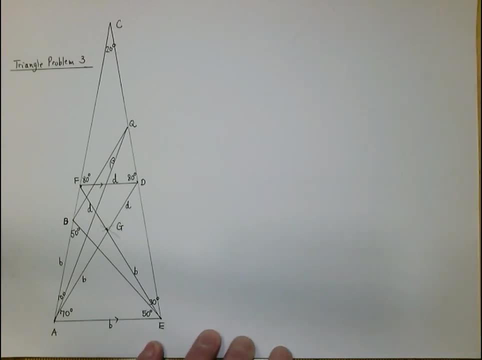 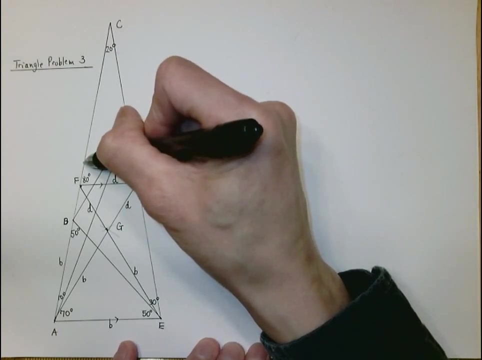 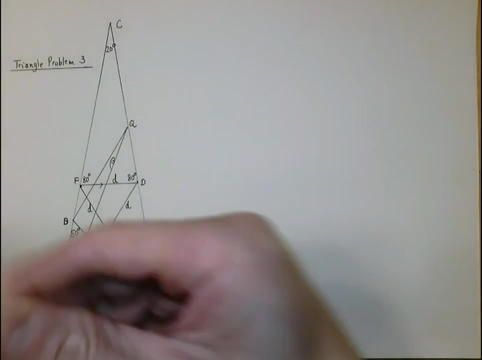 And that is also 80 degrees as well. Well, the next thing I would like to do is I'm going to locate a point Which I call H On CA, such that HA will be congruent to AD, And I'm going to use a compass to construct that point. 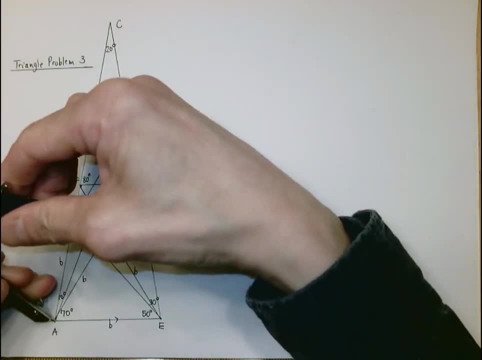 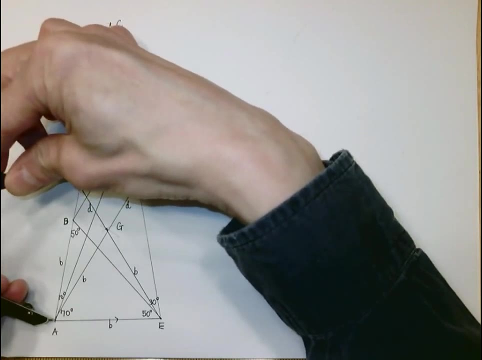 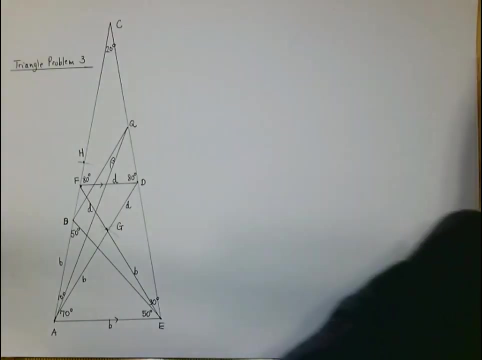 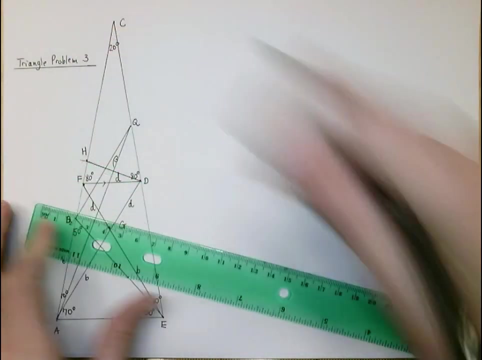 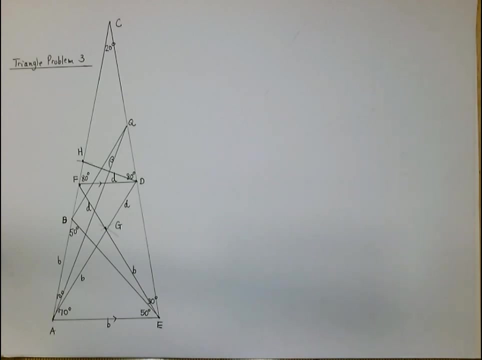 I'm going to measure AD And construct the point H. I'm going to call this point H, I'm going to connect H to D. And now I would like to focus on two triangles here: The triangle on the top And the triangles on the bottom. Well, I'm going to put in what we know here. 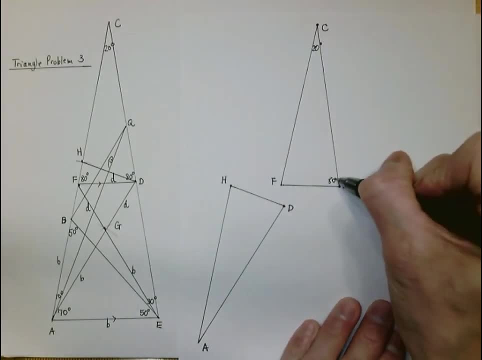 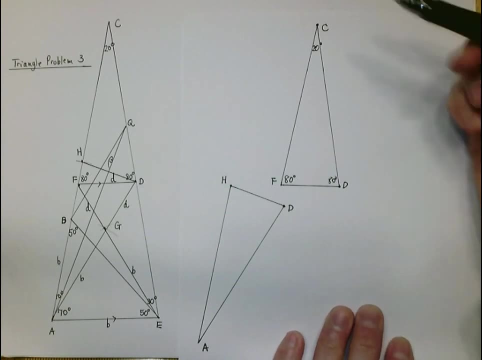 This is 20 degrees, This is 80 degrees, This is 80 degrees. So this is an isosceles triangle And we're going to look at this big triangle here From A to D to C. This is also isosceles because this is: 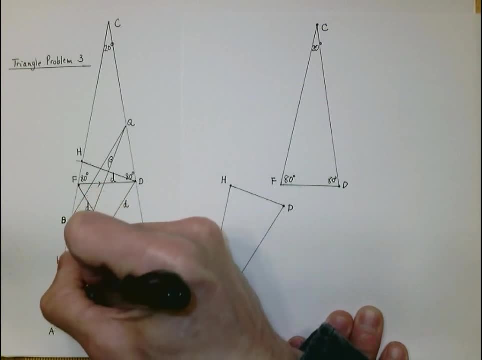 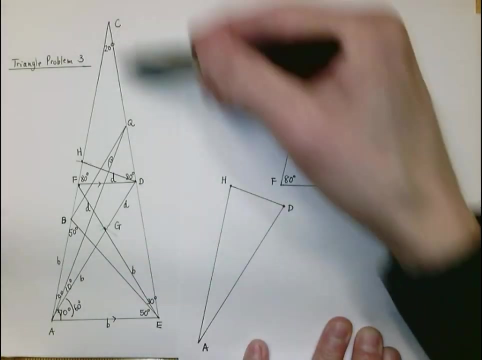 That is, I mean From here to here, is 60 degrees, But this big angle is 70 degrees. That means that is 10 degrees, So 10 degrees, and 10 degrees is 20 degrees, So that is an isosceles triangle. From A to D is B plus D. 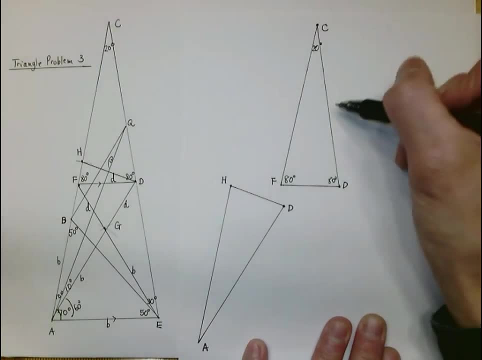 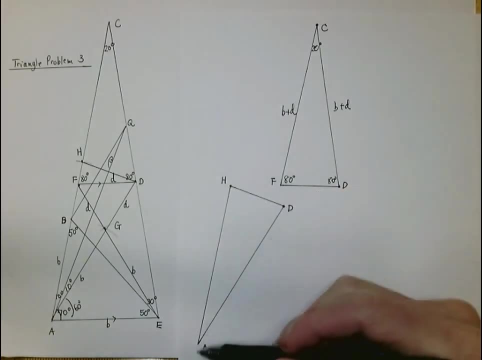 That means that from D to C would be B plus D, And that is B plus D as well. Well, we're going to look at the triangle here. Well, we're going to look at the triangle AHD here. AHD, We know that it is 20 degrees. 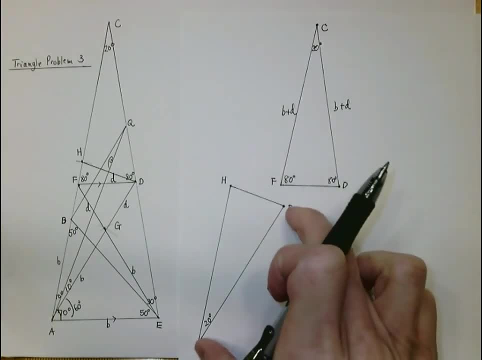 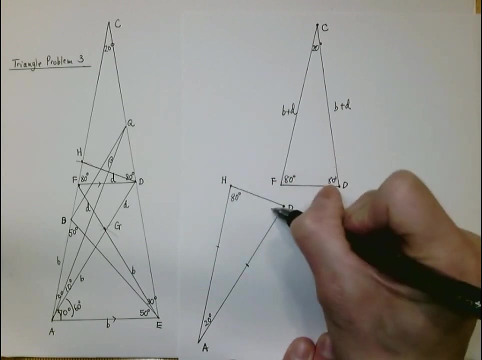 And it is Well based on construction, Based on our construction. HA is congruent to AD, That is isosceles. That means the sum of these two angles is 160 degrees. That means they must be 80 degrees each And we know that from A to D. 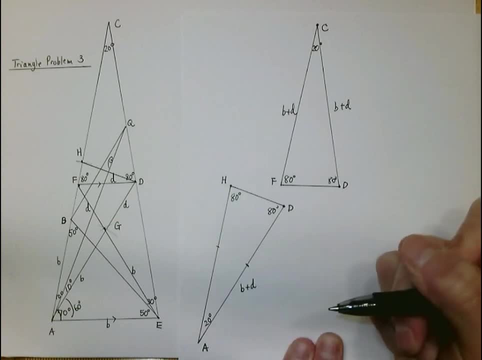 Is B plus D, So B plus D on the other side as well. So we can see that these two triangles are actually congruent: Side angle side, Side angle side. And the segment across from the 20 degree angles Must be congruent And we know that from F to D is small d. 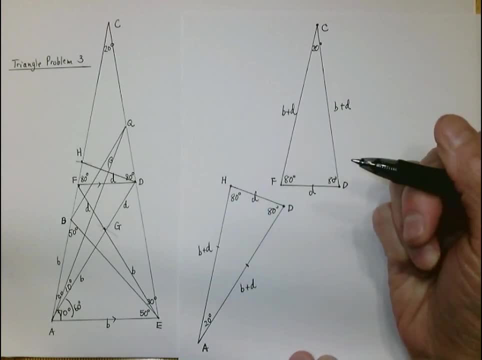 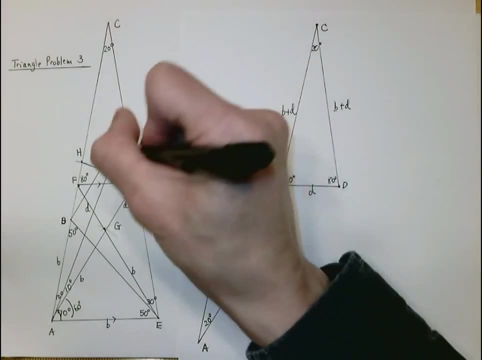 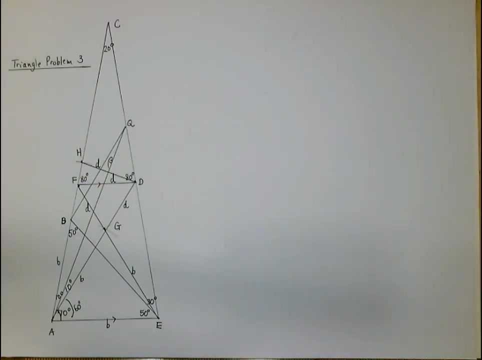 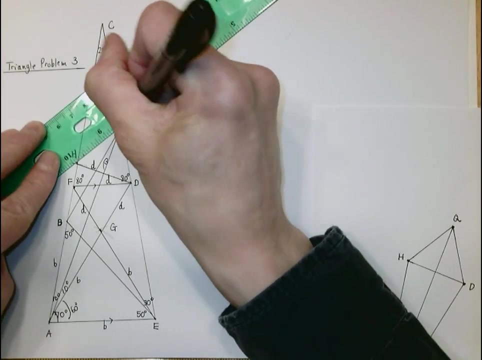 So this one will be small d as well. From F to D is small d, So from H to D must be small d, So this is small d. Let me put it over here. Well, the next thing I would like to do is I'm going to connect H to Q. 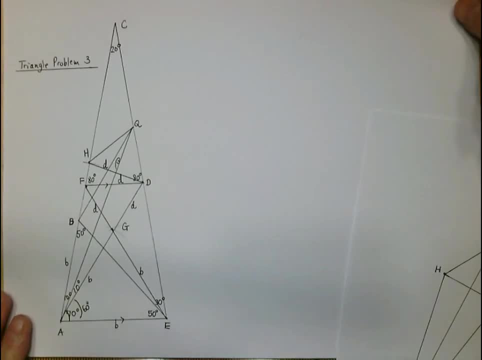 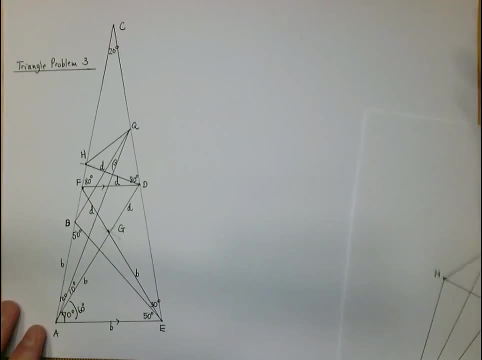 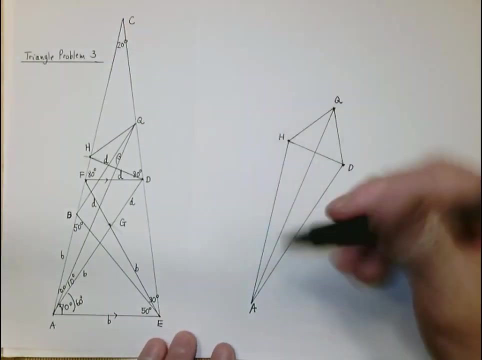 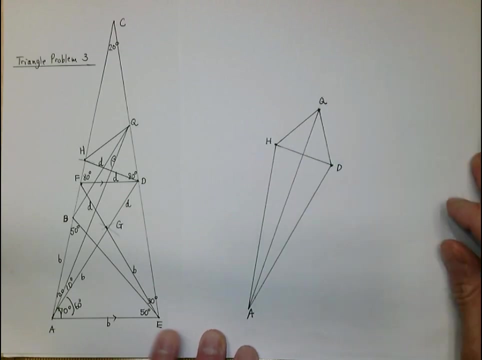 And I would like to show that. I would like to show that this triangle here, HQD, is actually another equilateral triangle. Well, here we go, I'm going to pull out the quadrilateral here. AHQD, AHQD. I pull this out. I'm going to put in the information that we know. 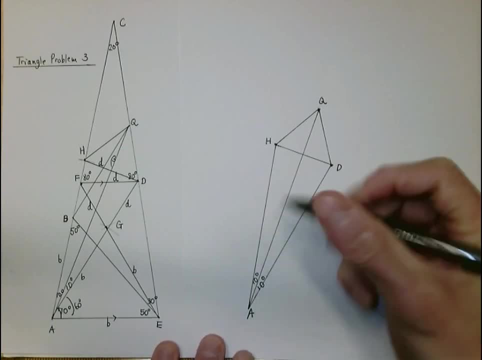 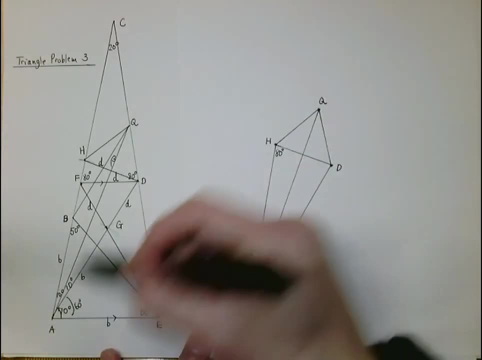 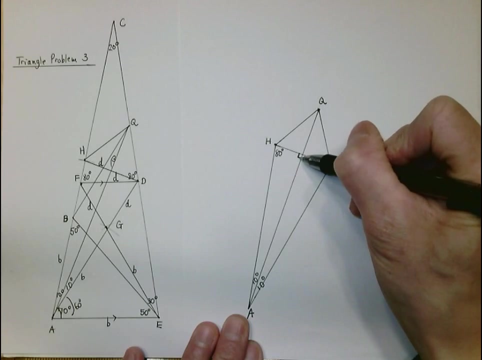 That is 10 degrees And that is 10 degrees And that is 80 degrees. Remember, that is 20 degrees, That is 80 degrees And that is 80 degrees. Well, 10 degrees, 80 degrees, Then that will make this a 90 degree angle. 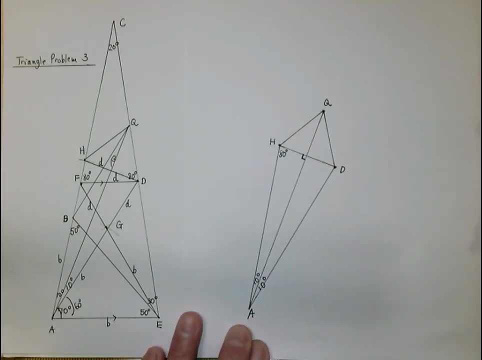 Because the sum of the three angles of a triangle Is always 180 degrees, When we have 80 degrees here And 90 degree angle. So these two triangles, These two triangles here, Must be congruent By angle. side angle. That means these two segments Are congruent. 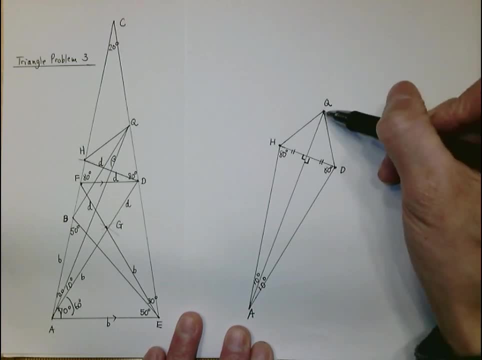 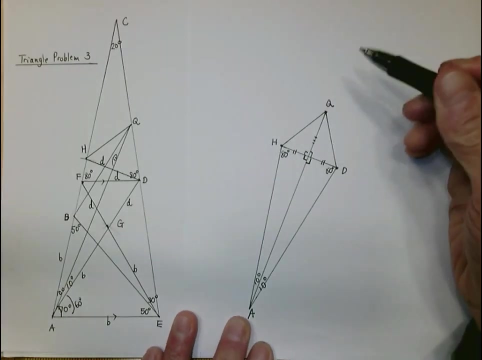 Well, look at this segment here. This segment is- I'm going to look at these two triangles here. This segment is A common side to both triangles And that is 90 And that is 90, So I would say that these two triangles Are also congruent. 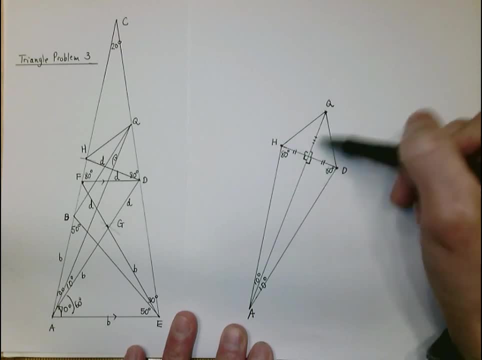 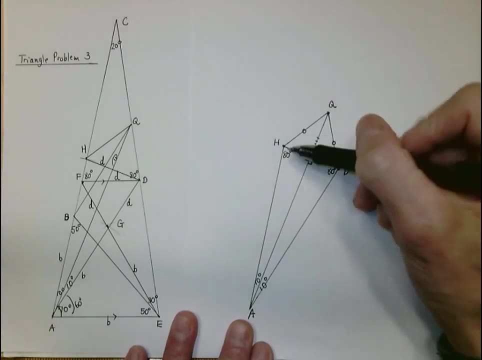 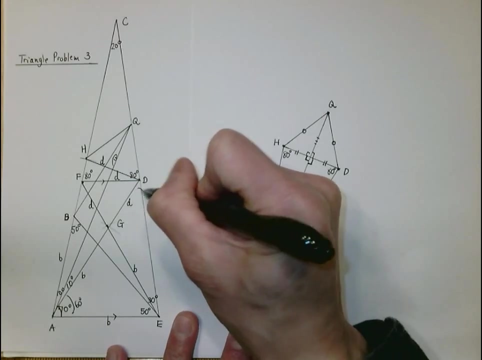 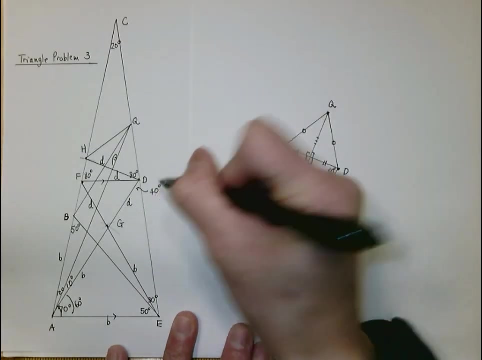 By side angle side, Side angle side. In other words, HQ must be congruent to Rd. I mean, HQ Will be congruent to Qd. Well, I'm going to look at this angle here. This angle here, I would say, Is 40 degrees. Well, that is 60 degrees. 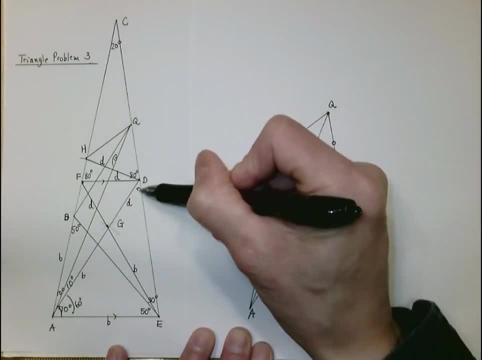 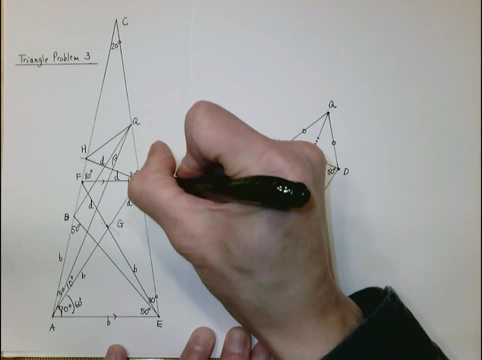 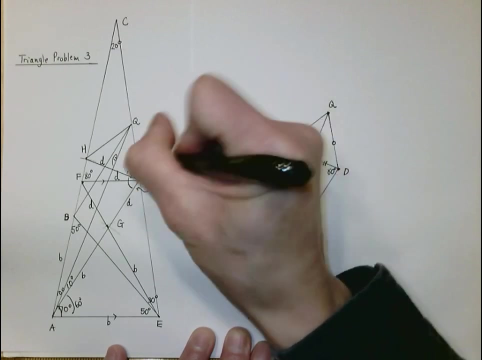 And that is 80 degrees, So this one has to be 40 degrees. The sum of the triangles, of a triangle is 180 degrees And this angle here Is 80 degrees. We know that 40 and 80, So this angle here Must be 60. 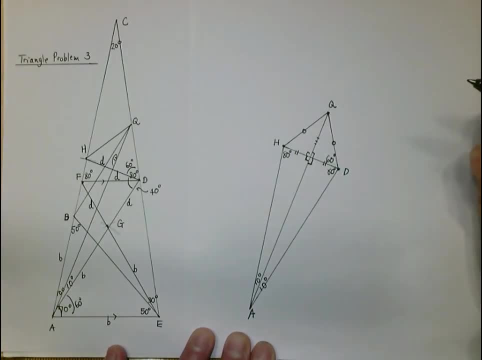 So this angle must be 60 degrees, But this is an isosceles triangle: If this is 60, This one will be 60 And that one will be 60 as well. So we actually did this. It is an equilateral triangle here, But we know that from H to D. 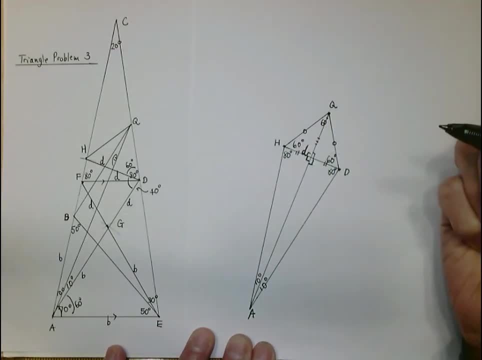 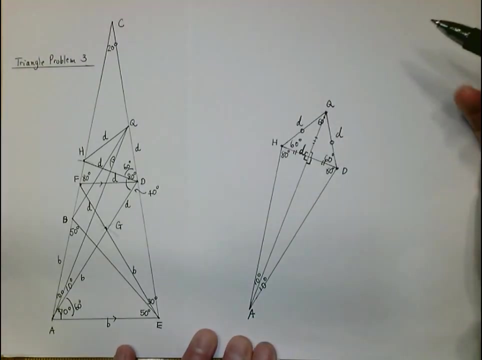 Is little d, Small d, So that means Qd And Qh Will be small d as well. So I'm going to put it over here: This is small d, This is small d, So Let's summarize what we have so far. Well, this is an equilateral triangle. 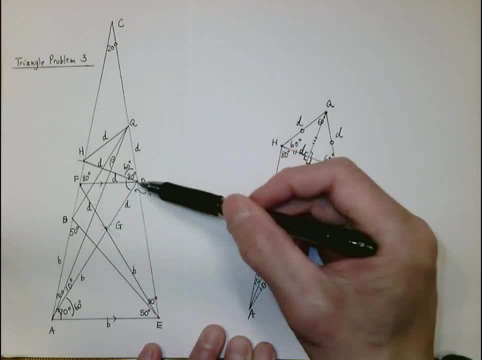 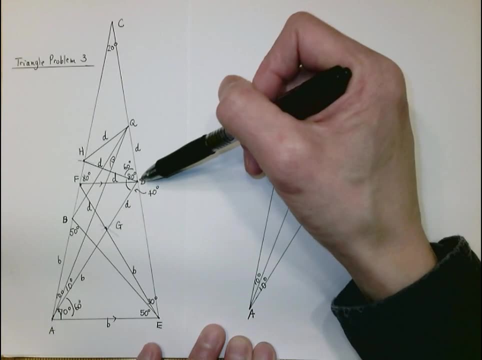 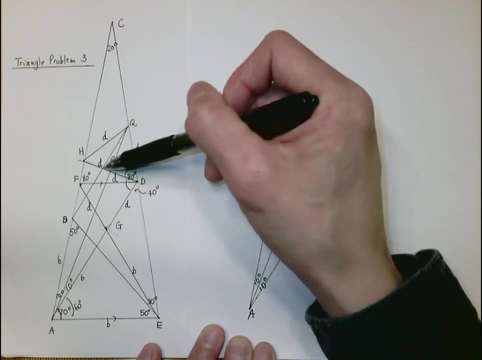 d, b, b. It is also an equilateral triangle And we call it d, d and d And we have just shown It is also an equilateral triangle. It is small d, Small d And small d. I'm going to reflect this triangle: H, b, q. 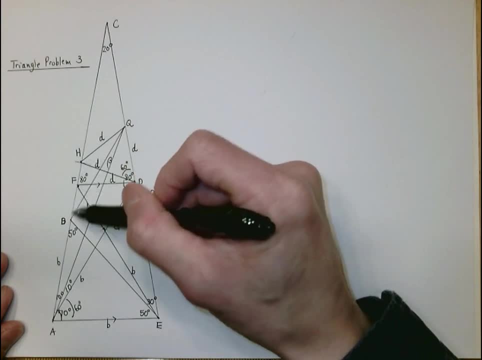 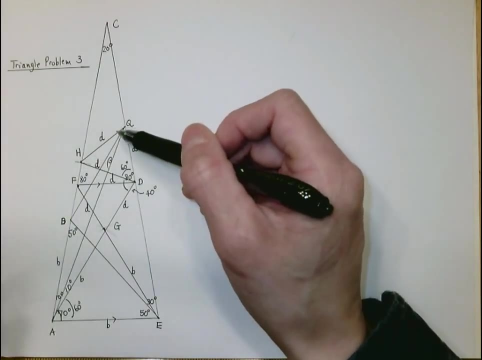 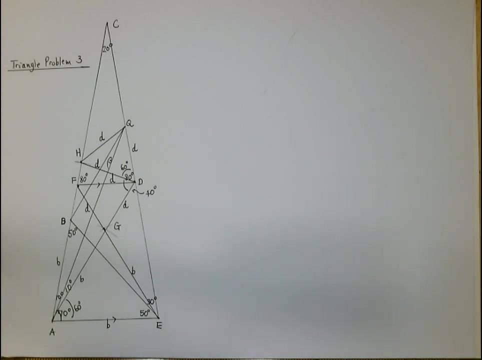 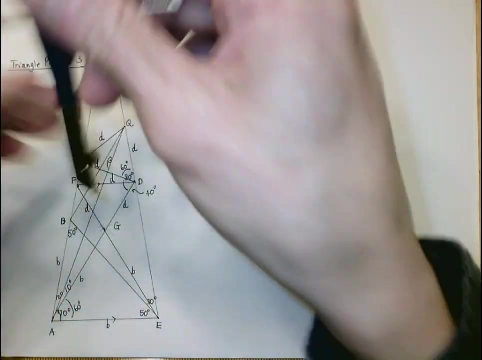 This triangle, Reflect this triangle along H b. I make a reflection, I make a copy of this. But on the other side of H b, And that is not difficult to do, I'm going to measure H q. I'm going to use a compass to measure H q. 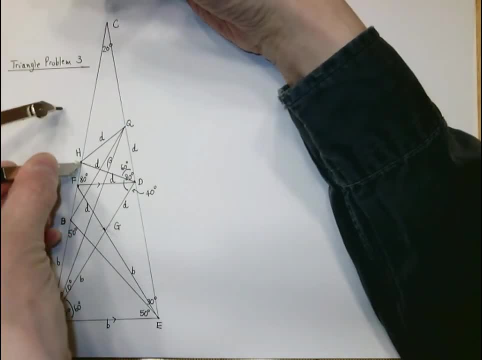 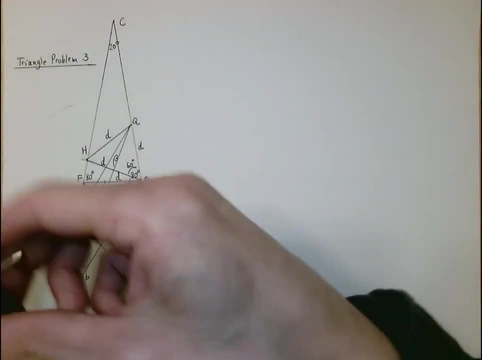 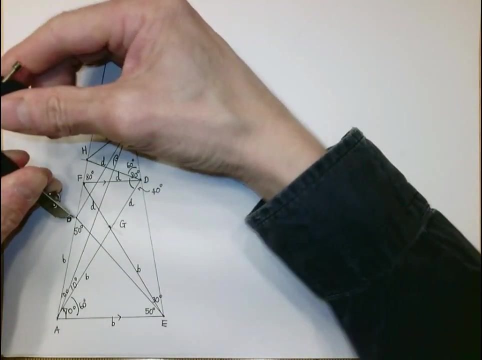 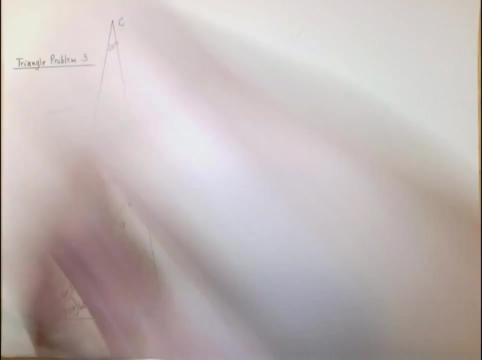 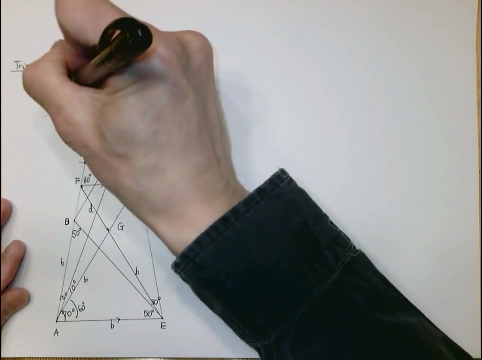 I make an arc here And I'm going to measure b q as well. I'm going to measure b q. I'm going to make another arc And I'm going to call the intersection point R. I'm going to call this point R. I'm going to call this point R. 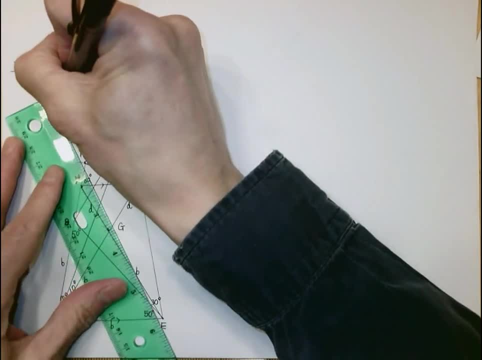 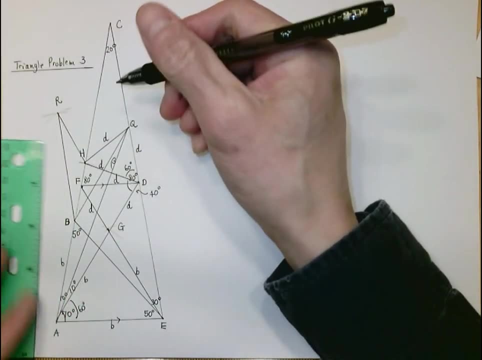 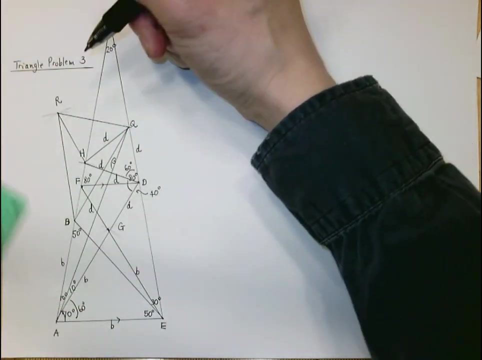 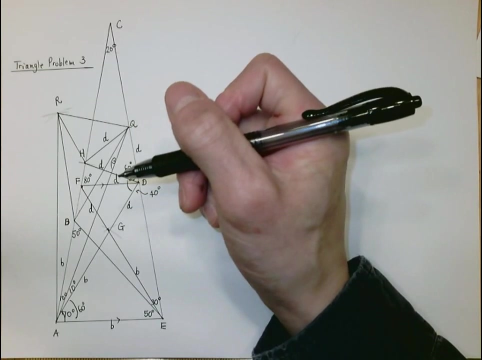 I'm going to connect H2R, I'm going to connect H2R, I'm going to connect H2R And I'm also going to connect E2R And connect Rq, And I'm going to connect A2R as well. Well, basically, I just make a reflection. 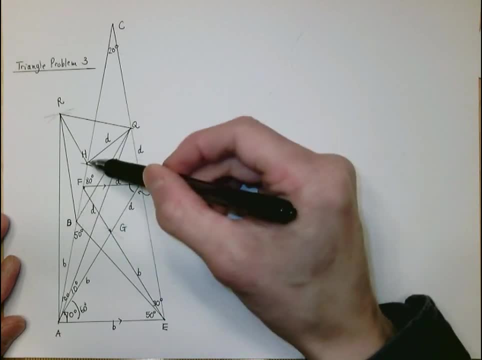 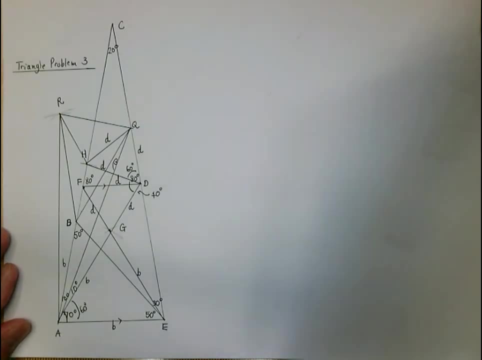 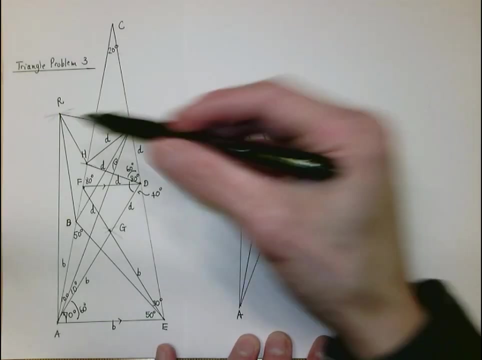 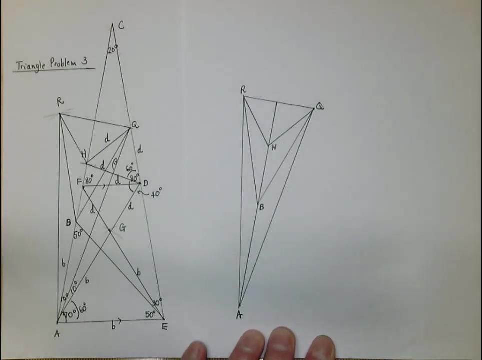 I make a copy of HBQ, but on the other side of HB. Now the next thing is: I want you, I want to focus on this triangle here: RQA, RQA, here, and we're going to write down what we know Based on the construction. we know that based on the 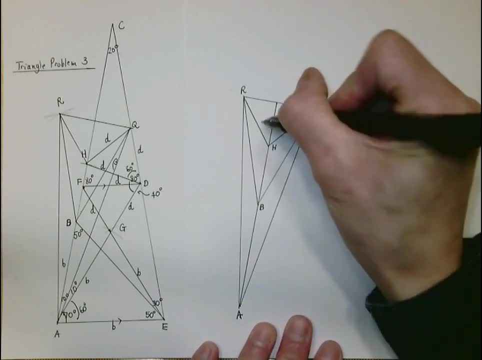 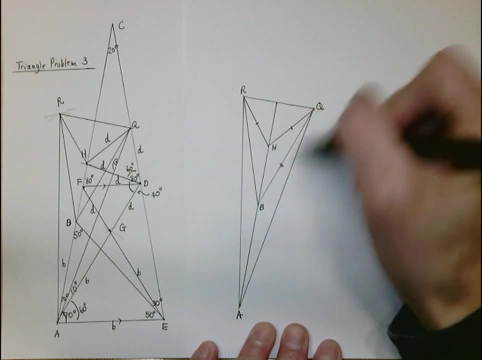 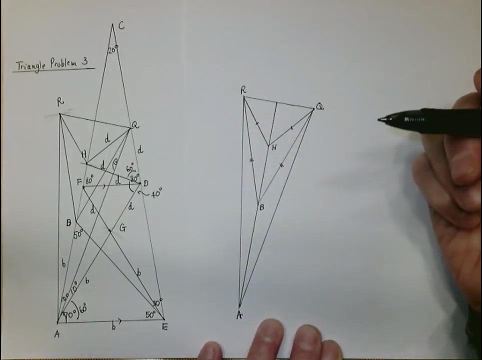 construction. we know that HQ is congruent to HR and HQ is congruent to, I mean, VQ, congruent to VR. Well, these two triangles here, these two triangles here, are congruent because we have side-side-side situation, side-side-side. so 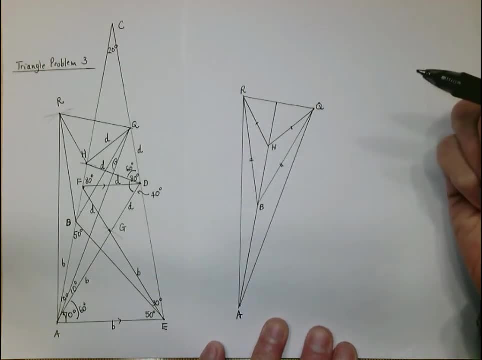 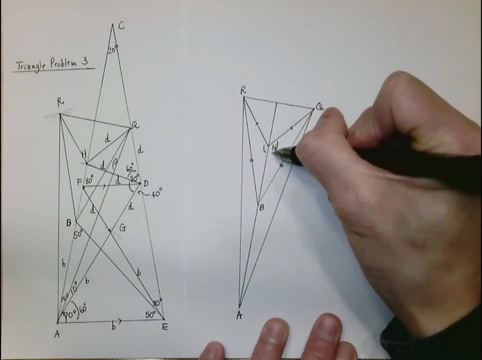 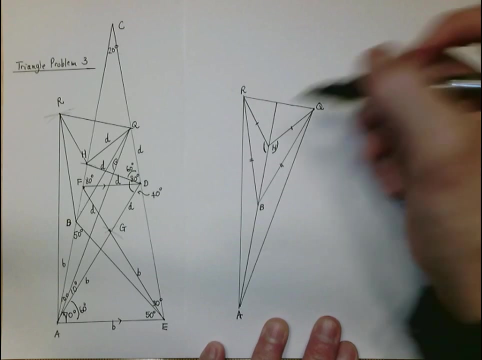 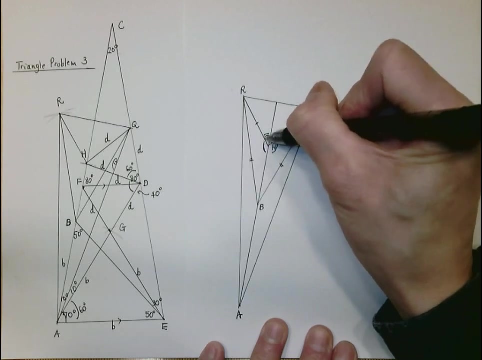 these two triangles are actually congruent. Let me write down again. so this angle and this angle are congruent. that means this angle and that angle are the same, They must be congruent. but look at this angle here. This angle, the sum of these two angles is 180 degrees, and the sum of these two 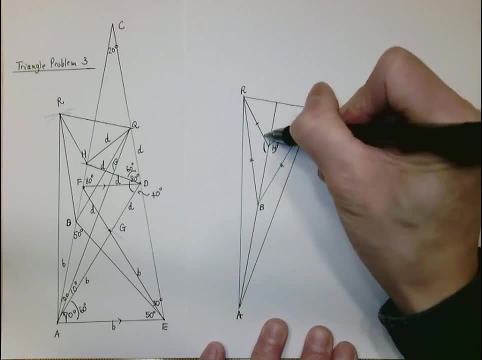 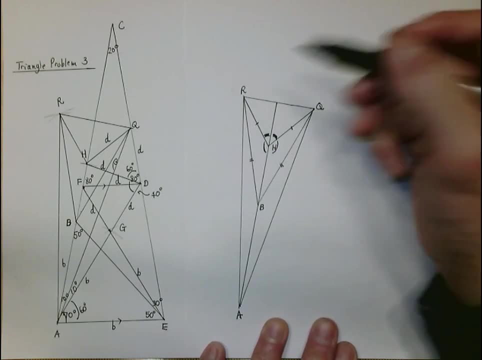 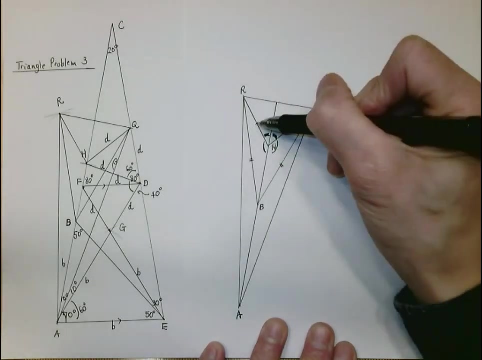 angles are 180 degrees, But these two angles are the same. that means these two angles here must be congruent And that will make these two triangles. that will make these two triangles congruent by side angle side, side angle side. 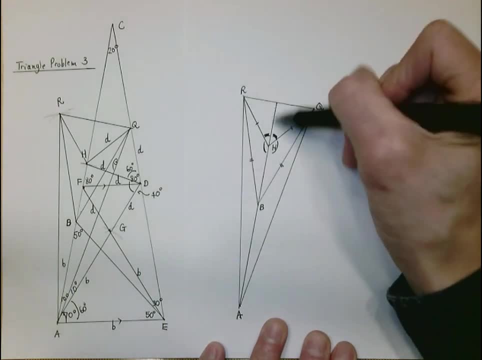 These two triangles are congruent, The one on the left and the one on the right, And that will make these two segments congruent And these two angles congruent as well. This angle here and this angle is congruent, But together they make 180 degrees. That means each one of them must be 90.. 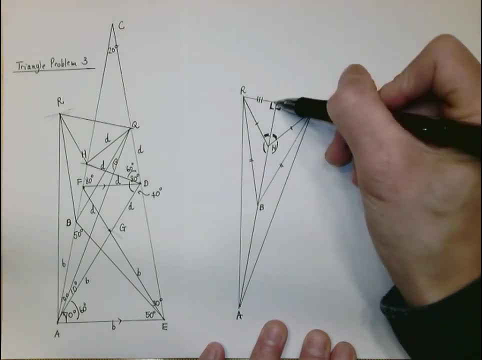 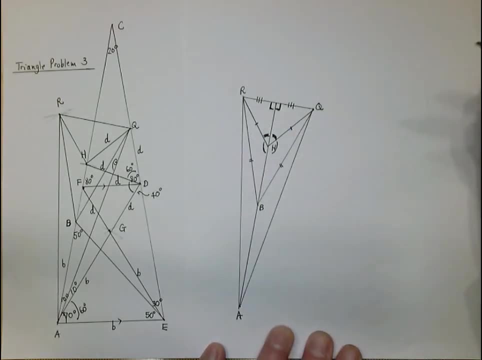 And now we're going to look at this big triangle here, The big triangle on the left and the triangle on the right. Well, again, they are congruent. The reason is quite simple: Side angle side, on the left, Side angle side. 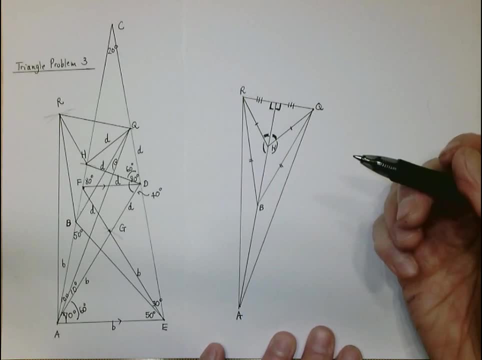 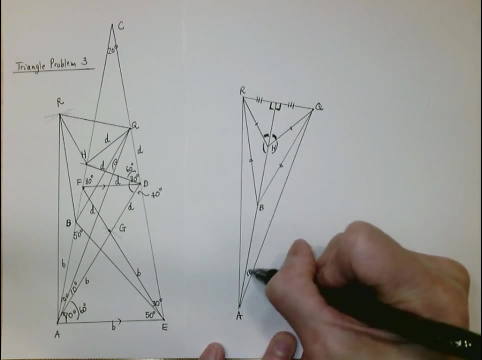 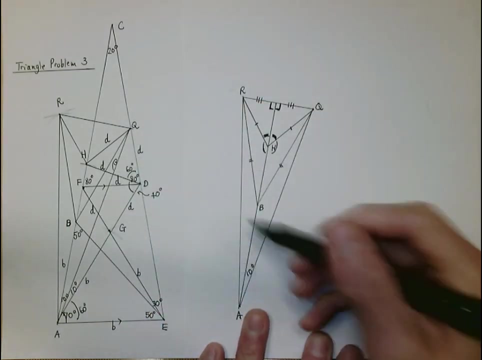 So we have a lot of congruent triangles here, But we know that this is 10 degrees. This angle is 10 degrees from the original diagram, But these two triangles are congruent, These two big triangles here. So that is 10 degrees as well. 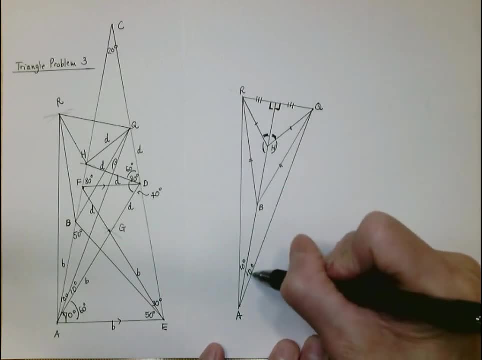 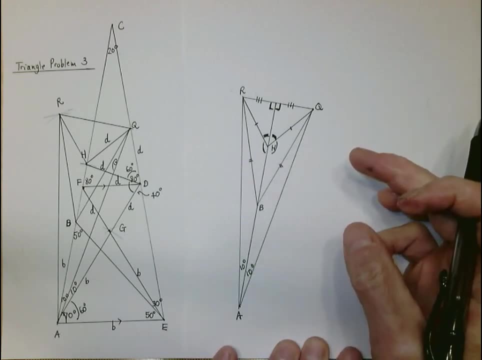 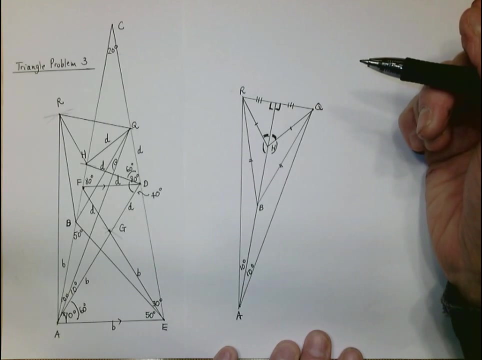 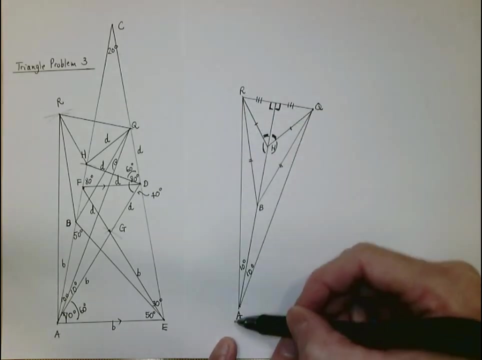 Well, 10 degrees and 10 degrees, that is, 20 degrees, Since these two triangles are congruent. Since these two triangles are congruent, Since these two triangles are congruent, AR will be congruent to AQ, AR will be congruent to AQ. 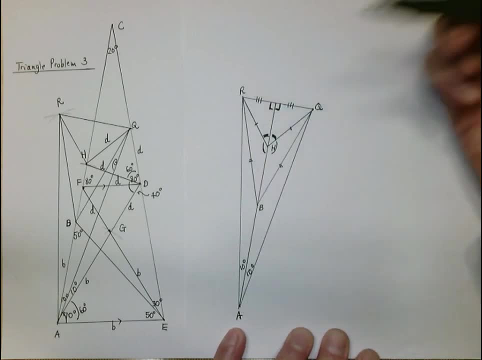 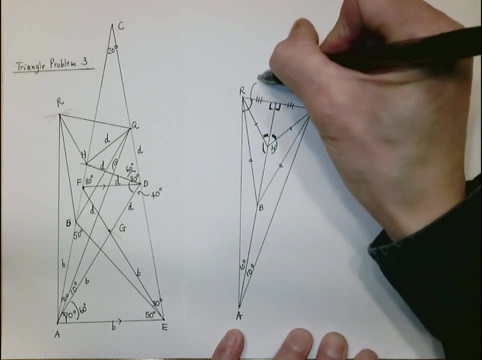 And that means it is an isosceles triangle, And that means it is an isosceles triangle. So this big angle here Would be 80 degrees, Would be 80 degrees. That is what we know so far. That is what we know so far. 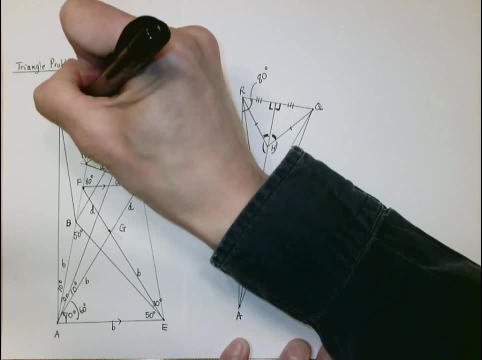 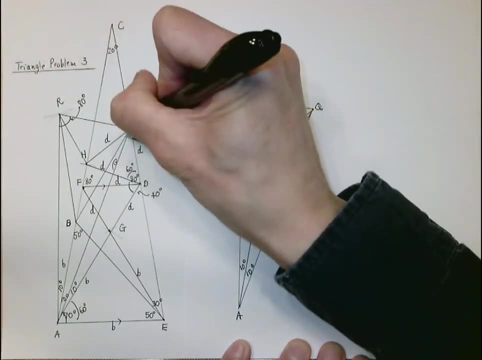 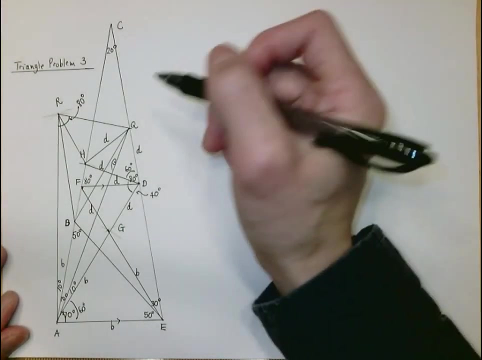 So that is 10 degrees And this angle here And this angle here Is actually 80 degrees, And the same thing over here, That is 80 degrees. Well, Based on the construction, We know that HQ Is congruent to HR. 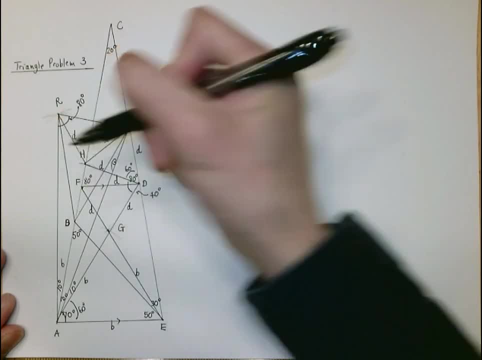 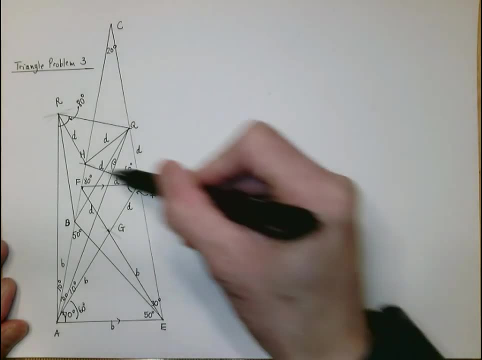 But HQ is small d, So this one is small d, And now we want to look at this triangle here. And now we want to look at this triangle here. ADH is an isosceles triangle. ADH is an isosceles triangle. 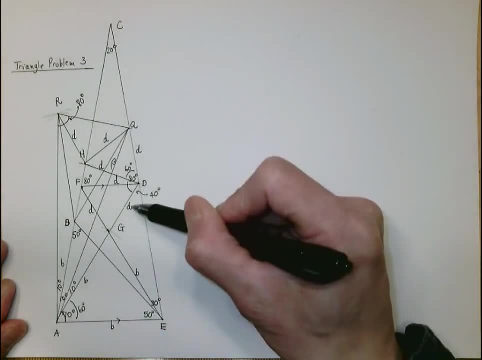 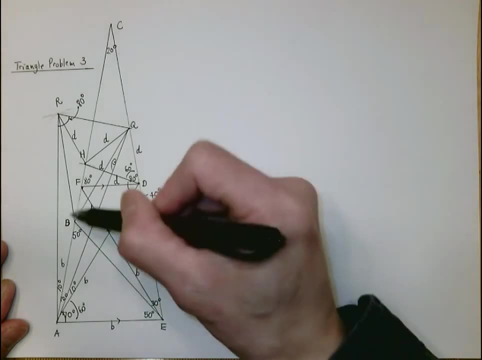 From A to D. That means from A to H. That means from A to H It is B plus D. From A to B is small b. That means that from B to H, From B to H, Will be small d as well. 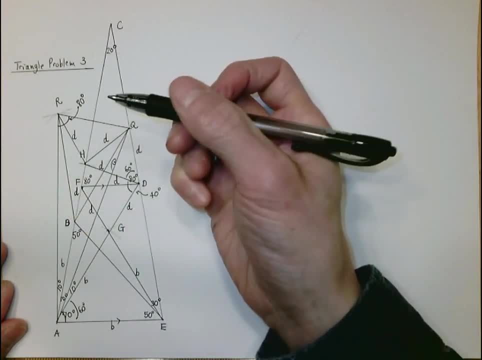 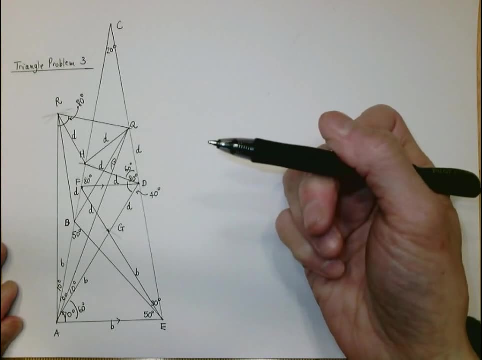 Will be small d as well, B plus D, B plus D On the left hand side And B plus D on the right hand side. And now I want you to look at this. And now I want you to look at this. 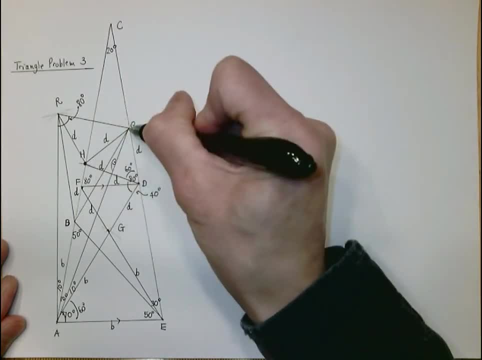 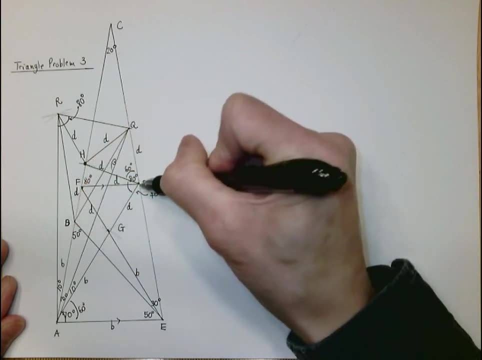 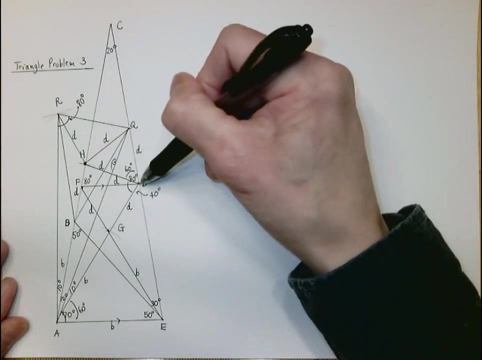 Look at this point: H From H to Q is small d, from H to R is small d, from H to B is small d and from H to D is also small d. That means that Q, R, B and D falls on a circle with center H. 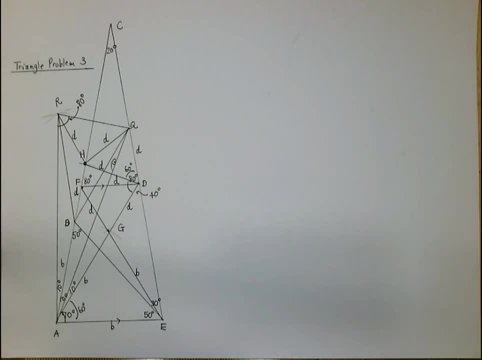 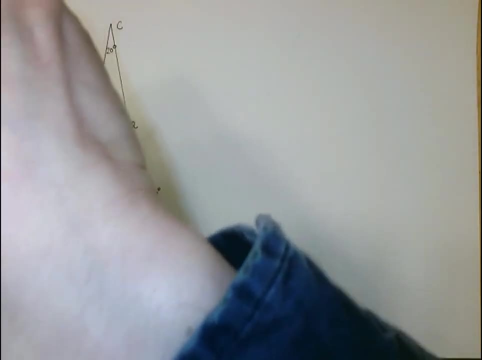 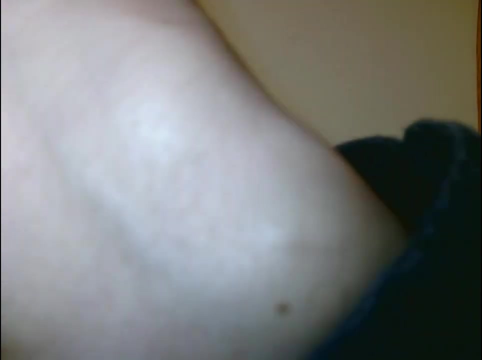 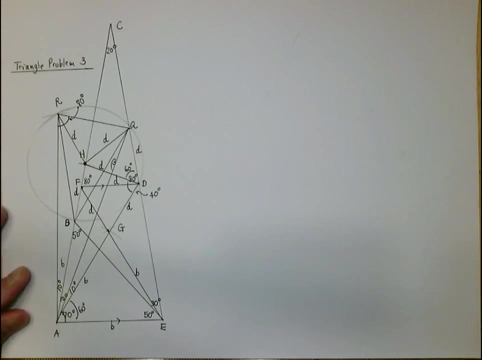 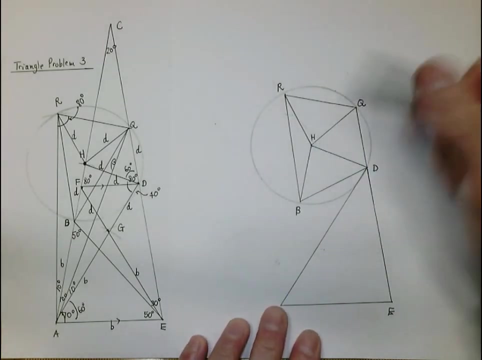 Actually we can construct that circle with center LH and we're going to make that circle. I have pulled out the circle here and it is the center of the circle H. And now I would like to look at this angle here, from B to D to A. 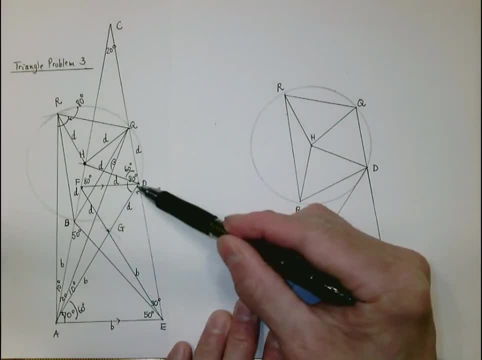 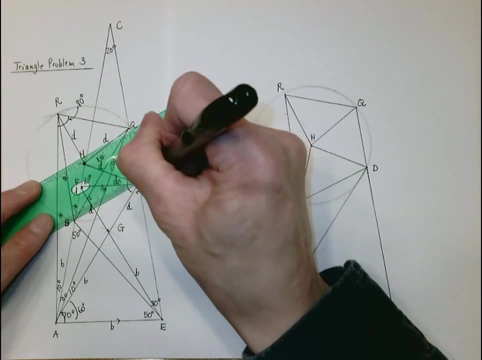 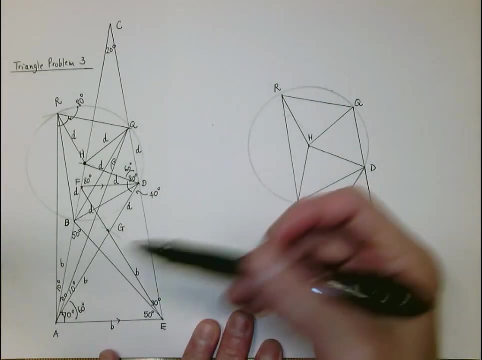 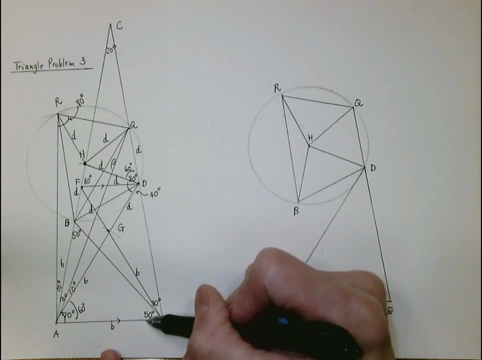 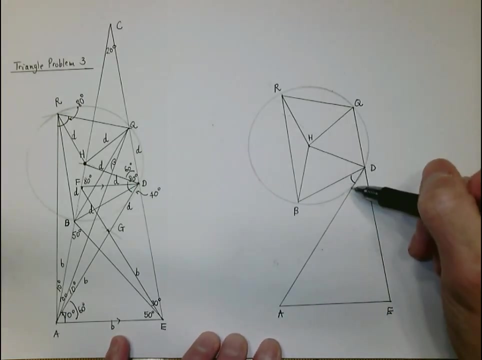 From B to D to A. Let me connect B to D, Okay, From B to D to A. Well, this is 60 degrees, This is 60 degrees, This is 50 degrees, And this angle is actually the unknown in triangle problem number one. 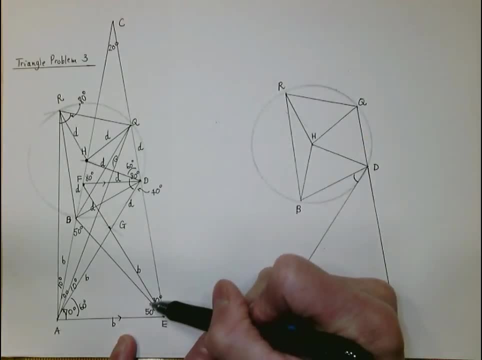 I hope you remember triangle problem number one. This is 50 degrees And that is 60 degrees, That is 60 degrees And we are looking at this angle And this angle is actually 30 degrees. We know that from triangle problem number one. 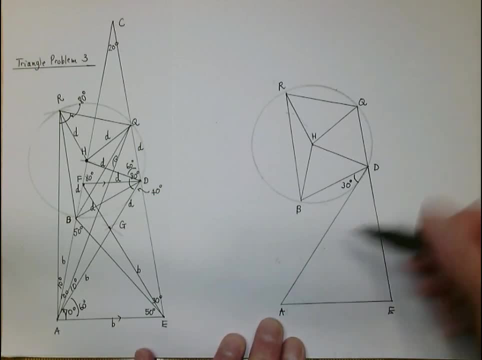 And we want to find out what is this angle here? Well, we know that it is 60 degrees. This angle here is 60 degrees and that is 80 degrees, 60 and 80.. That is 60 degrees, 60 and 80.. 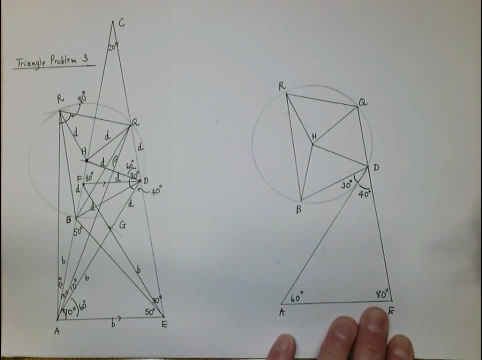 That is 140 degrees, And then we will make this angle 40 degrees. That means that we will make this big angle 70 degrees And then we will make this angle 110 degrees Because it is a straight angle here. But we know that, since this is a quadrilateral inscribed. 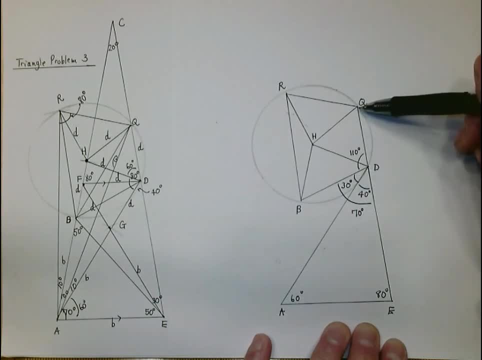 inside a circle. it is a well-known fact that the sum of the opposite angles of a quadrilateral inscribed in a circle is 180 degrees. So this is 70 degrees. The sum of these two must be 180.. So b r q from b to r to q is 70 degrees. 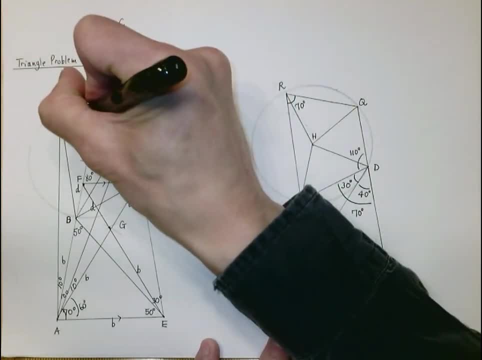 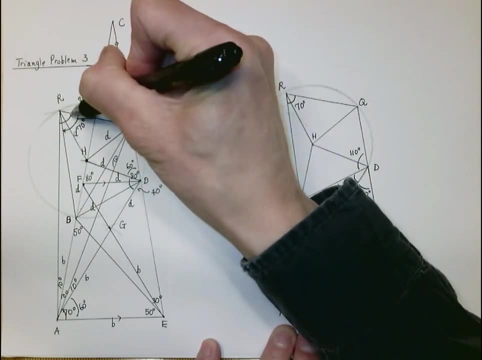 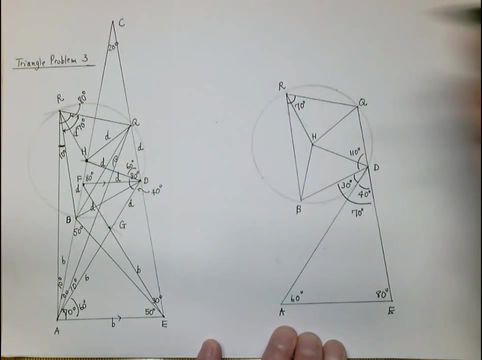 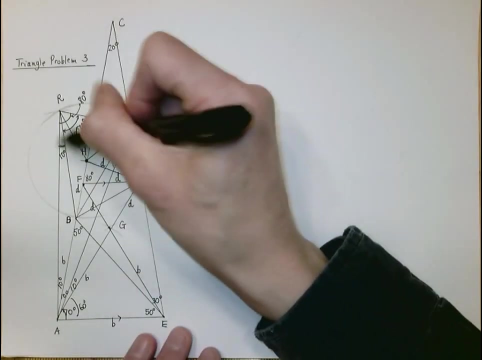 From b to r to q. this angle here is 70 degrees, But we know that this big angle is 80 degrees. That means this small angle here is 10 degrees. We are very close to solving the problem. If this is 10 degrees, this is 10 degrees. 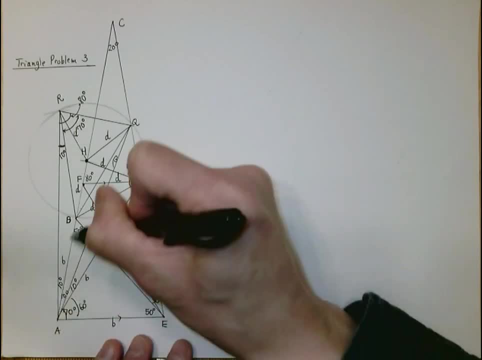 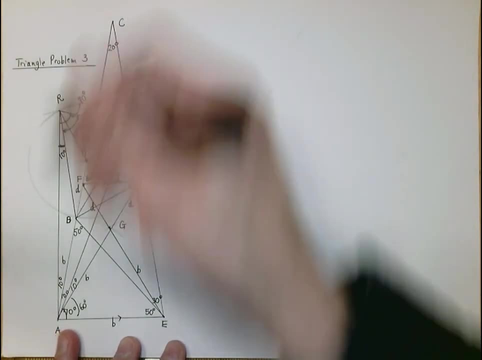 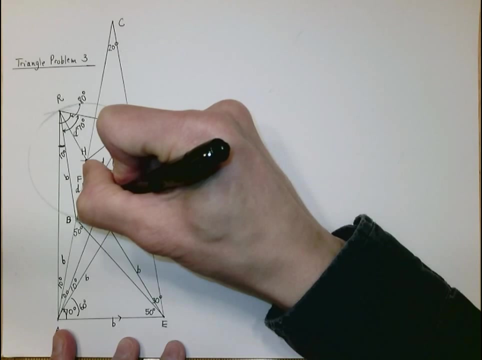 this is 10 degrees. so that will make this triangle here a b? r and isosceles triangle. But we know that from a to b is small b. That will make b? r small b. Well, small b here, small b here. 10 degrees and 10 degrees. 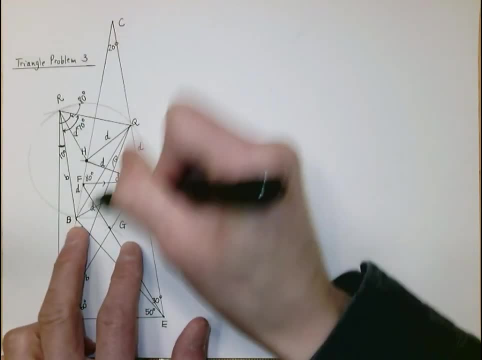 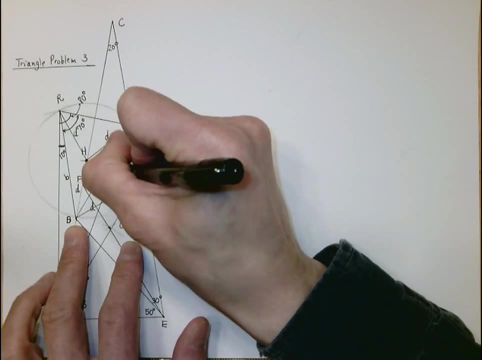 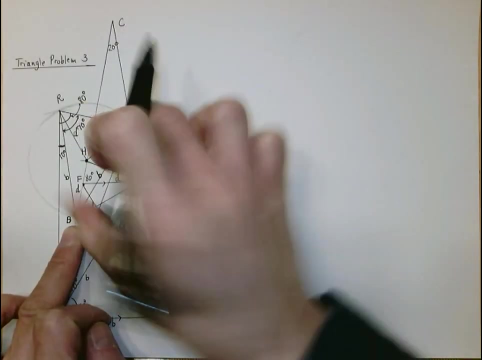 But b, r is small b and that will make b q, b q small b s, b q small b, Because this is how we construct, how we construct these two segments. So from b to q is small b. 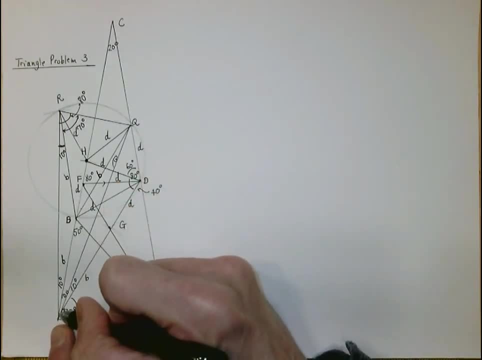 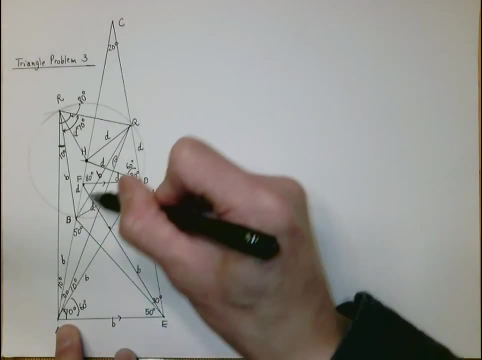 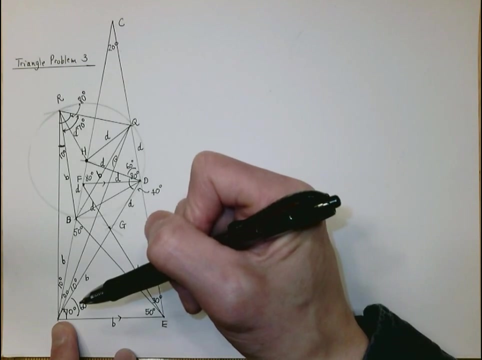 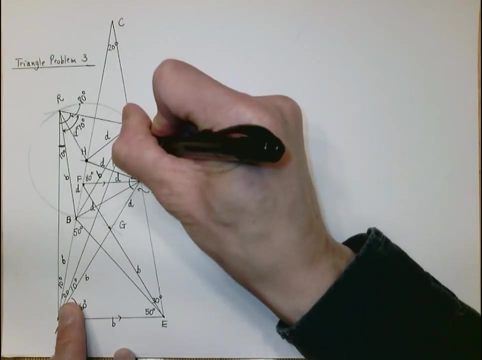 But from b to a is also small b. That means b q a. this triangle here b q a is isosceles, But this is 10 degrees And that will make this angle here again one more time. this is an isosceles triangle. 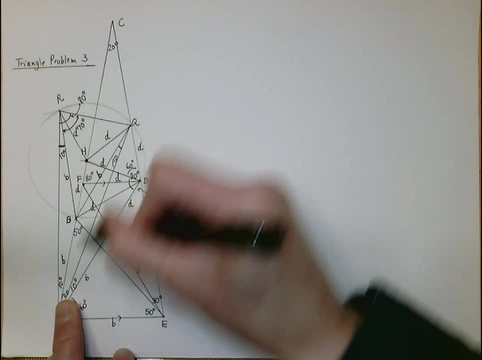 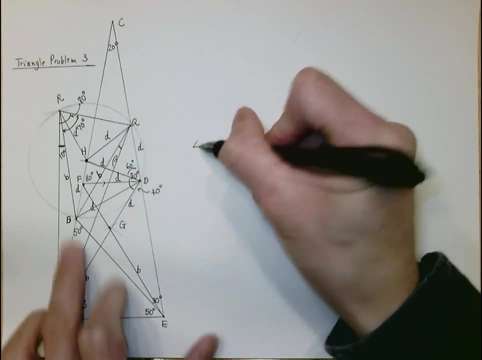 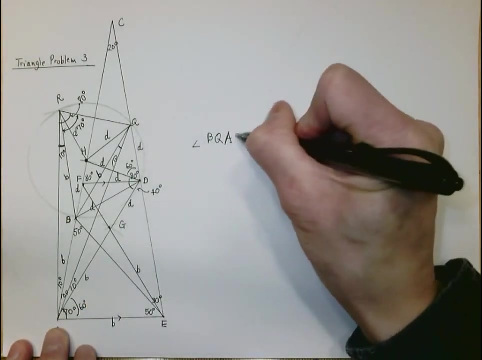 b here, b here. this is 10 degrees and that will make this 10 degrees, But this is the unknown. what we are looking for. We are looking for angle b q a. b q a is actually the angle beta. 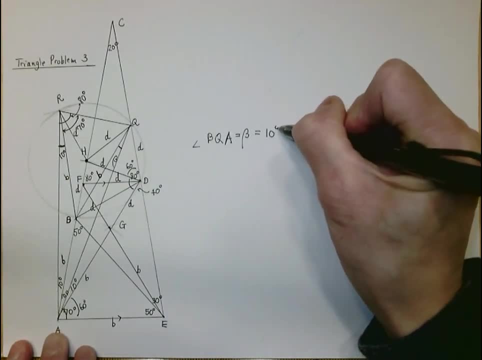 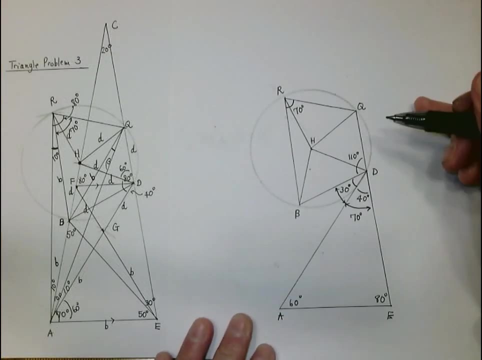 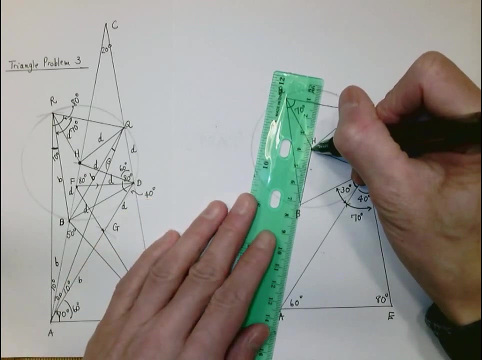 which is 10 degrees. I want to make an additional comment on why this angle has to be 30 degrees. Well, actually that is the problem from triangle problem number one, But I just want to make an additional comment. Well, we know that h, b, a is actually. 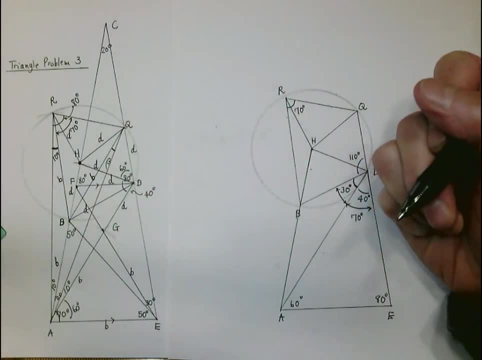 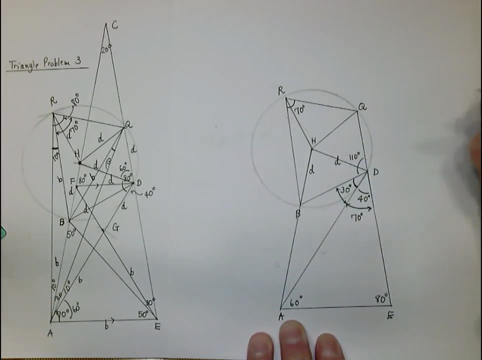 called linear. Well, we know that this is small d and this is small d, So this is an isosceles triangle, But we know that this angle is 80 degrees. Well, a, h, d, this is 20 degrees here. 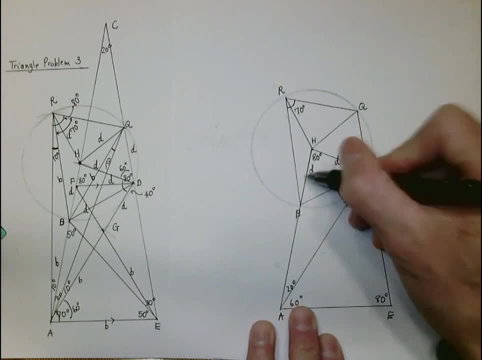 80, and 80 degrees, But this is an. well, look at this. this is an isosceles triangle, This is 80, and that will make this 50 degrees And that will make this angle 50 degrees. 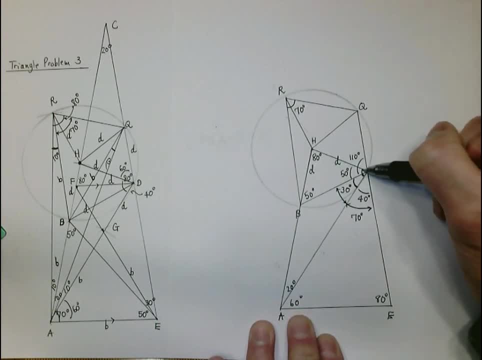 But we know that this angle here, this angle has to be 80. But this is 50. In other words, this one has to be 30 degrees. I think that may make it more clear to the audience why this angle is 30 degrees. 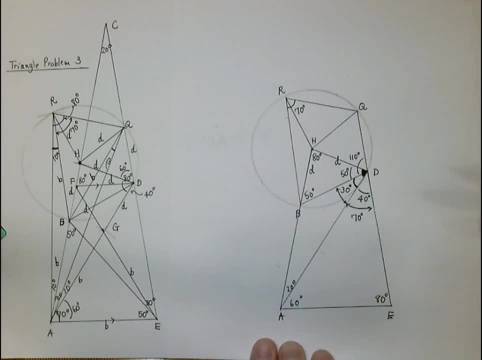 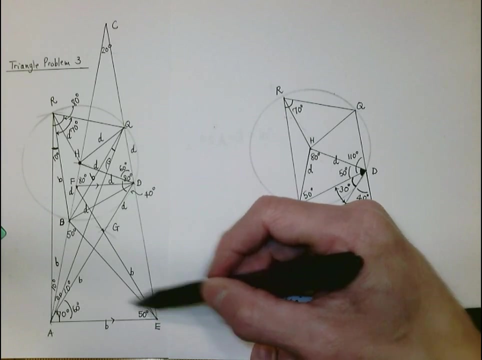 And actually that is triangle problem number one. And that concludes the solution for triangle problem number three. And in the next video we will talk about how to find a general formula for arbitrary isosceles triangle and arbitrary angles formed by the segments inside the triangle. 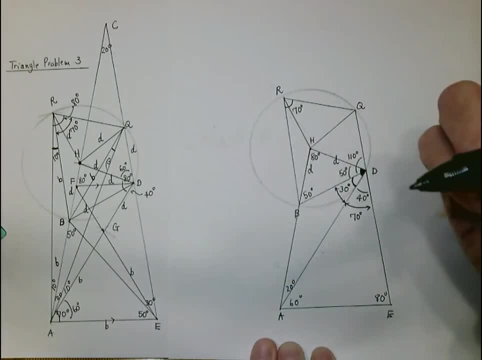 and the base of the triangle, And hopefully you will join me watching video number four. Thank you.